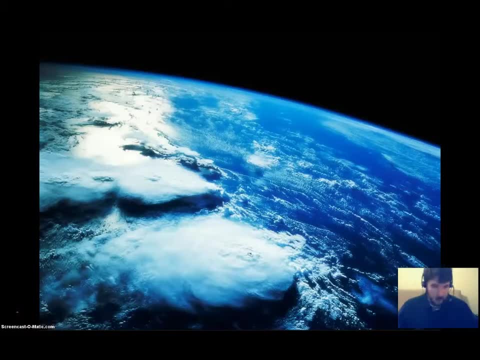 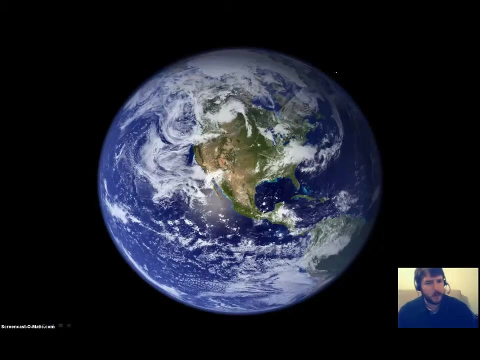 Well, hey, there, boys and girls, This is quite possibly the first flip class of the year and this one is all about the earth, which is, you know this thing down there. There it is, you know, being the earth. that's nice. As you can see from the picture here and the picture here, the earth is pretty much mostly water. You know, we got the United States of America there. it is being all you know America, But for the most part the earth is all covered in water. Now we're going to study a lot about the ocean, but to really understand the ocean and the 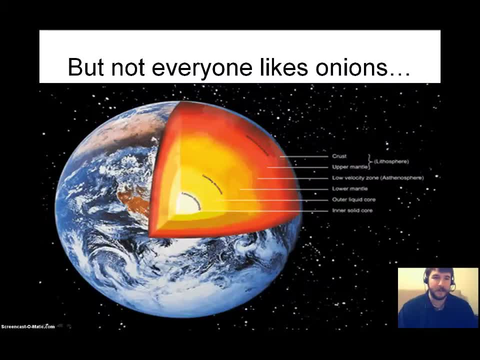 ocean floor. you have to understand the geological processes that are going on. So let's go ahead and dive into it. Remember the earth has many different layers. you know, just like Shrek does. You've got the crust and the upper mantle Now together. those often is called the lithosphere, which is technically just under the crust, that really top part of mantle that's still really hard and rock like Then below that you can see in this area. here you have the asthenosphere. Astenis is a really fun Greek word that 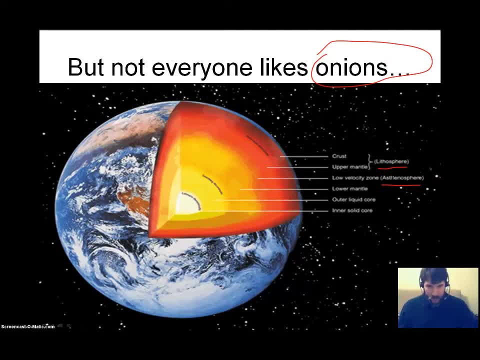 means weak. It's really weak, flexible, flimsicated and, just in general, unimpressive. Underneath that you have the lower mantle, which is also referred to as the mesosphere. It's got meso in it, because that is the word for middle, So that one right there. that's the mesosphere. Then you have the outer core and the inner core. Keep in mind that the outer core is sort of liquidy, It's just gooey and it's got flow to it. and later on we're going to 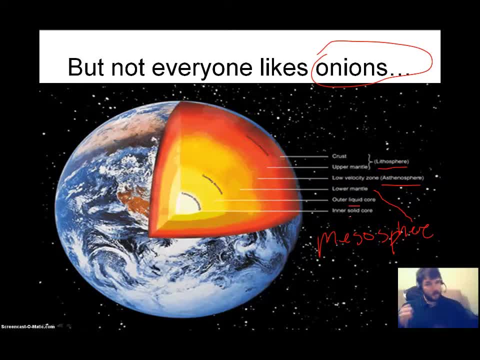 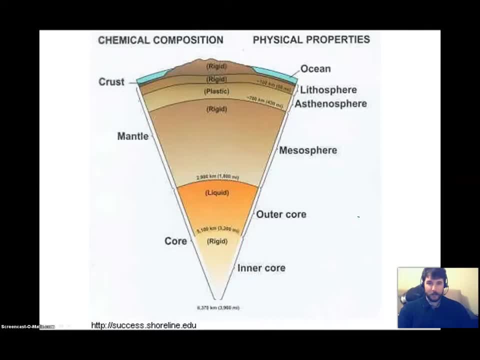 talk about why that's really important and what that actually does for the earth. I'll give you a hint, though. Turns it into a magnet And then you have the inner core, the solid area that's pretty much just spent from. you know the fusion that's been taking place inside the earth. So here in all its grainy goodness is the layers of the earth, And you see the cat that was trying to be in the video. That's kitten little. Right now he's down there playing with the dog. I'd move the webcam but it gets crazy. So you know you have the. 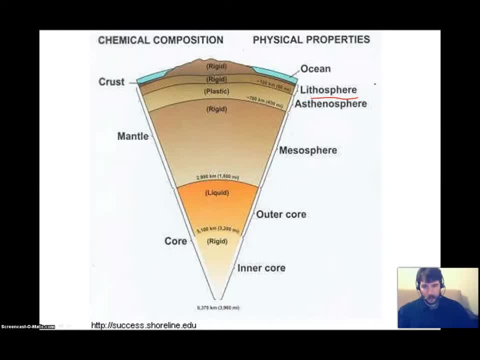 lithosphere. Again, we're going to talk about the difference between continental lithosphere and oceanic lithosphere in a little bit. But first let's just know it's lithosphere, asthenosphere. Then you have the mesosphere in the middle, Outer core, which is liquid, Inner core, which is rigid, It's worth mentioning. the asthenosphere is sort of liquidy. This mantle is actually very rigid, like they're saying right here, And there's some convection in there, But for the most part it's very stiff and rigid and hard. So now that we understand the layers of the earth, 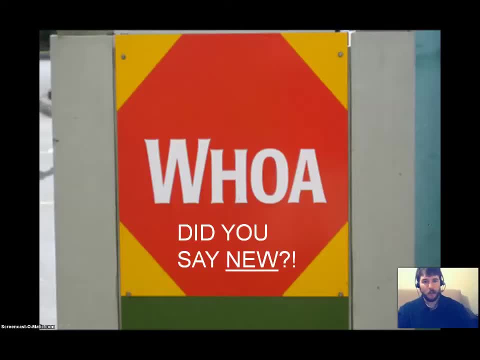 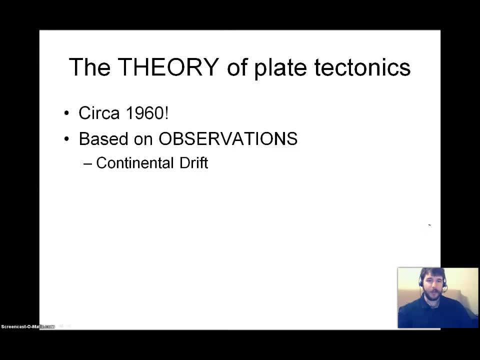 a little bit. let's get into plate tectonics, which is actually relatively a new thing. Plate tectonic theory really originated back in the 60s and is a pretty new thing. It's actually based on some observation. We got continental drift. you know Wegener's whole thing. Just he couldn't put a good mechanism with it- And we've actually seen continental drift, rebranded seafloor spreading, which was actually discovered by Captain Henry Hess, a US Navy captain, back in WW. 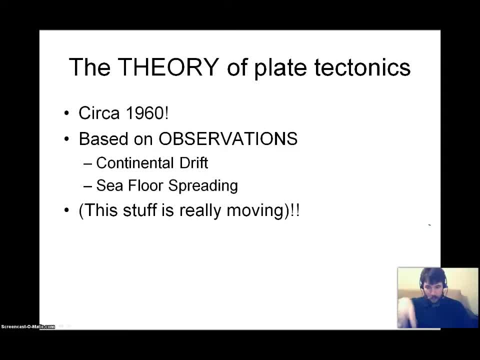 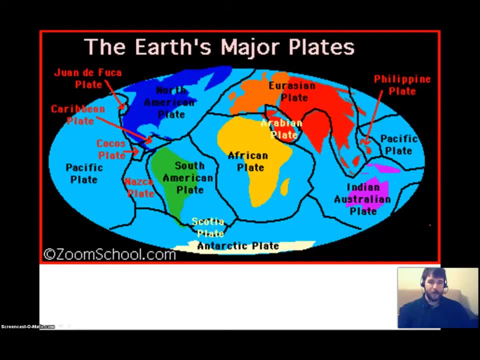 Dose. He was just floating around looking for the German U-boats, pointing his pointer down at the bottom of the ocean, which was looking at all the things he saw on the ocean. And so we have the earth. It's made up of these main plates. There are more little plates that are hanging out in there around there, And you know we won't really care too much about them though, But these are the main plates. I'm not going to make you memorize them. That's what books are for, But you should probably know that the North American plate is where North America is, The South American plate is where South America is, The African plate is where South America is. 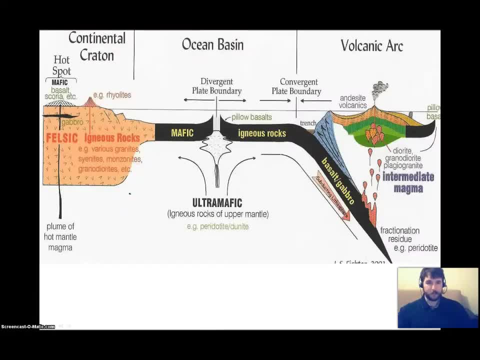 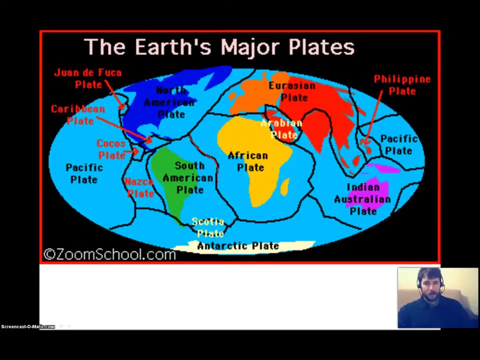 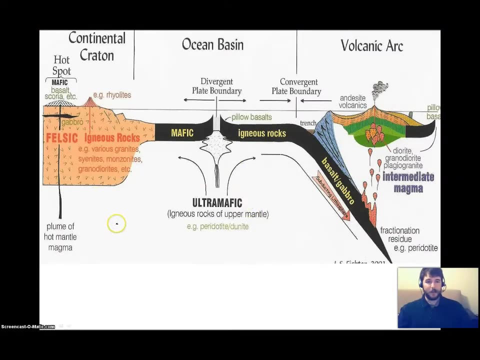 Well, you can see the pattern: Pacific plate- That's a big old ocean. So those boundary lines in between that we were showing here, These lines are the spaces in between the plates and we call those the plate boundaries. There's three basic types of plate boundaries: You have convergent, divergent and transform boundaries. This is a picture that's showing you the middle of the ocean- size, continents, and you can actually see that we've got a nice divergent. 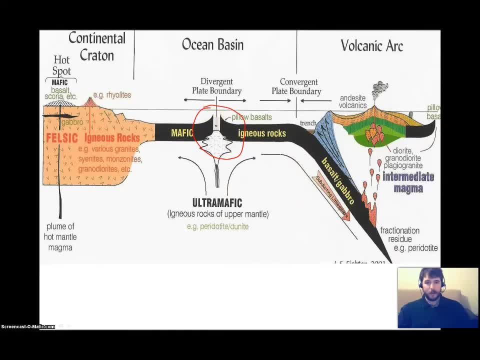 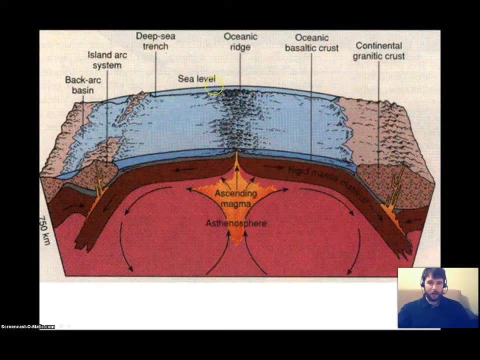 boundary here with the spreading center in the middle And then over here on the side. you can see that we have a subduction zone going down. Subduction And that is a convergent boundary where they're coming together. Here's another one showing you you have in the middle, you have your spreading center, Creates all kinds of really fun stuff on the surface, like mid-ocean ridges etc. We'll get more into that a little bit later in the unit. 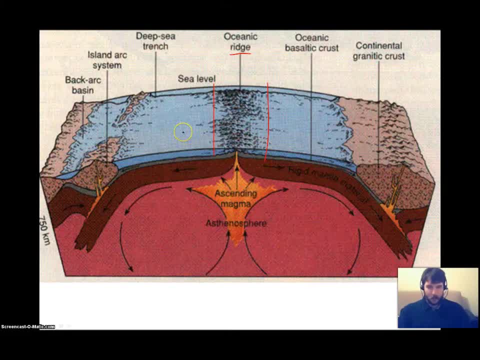 But again you have these divergent boundaries where you have this plate is moving in this direction and this plate is moving in this direction, so they're diverging away from each other. Now what happens is when the plates here run into the next plate over, here is the plates come together, you get a subduction zone and you have a convergent boundary, And all this is generated is because of this whole mid-ocean convection thing. So you can see, here we've got this. 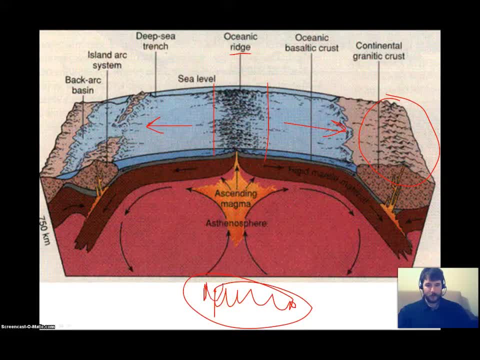 area down here where it's hotter. See, that's the flames for heat And it gets hotter and that causes things to rise And then, as they rise, they come up towards the surface where they interact with that rigid lithosphere And it sort of spreads off to the side. Again, this is all happening in the asthenosphere. The idea with a lot of people is: this all goes on down in the mesosphere, But not so much children. Instead it's happening in the asthenosphere and you get these convection currents just like a 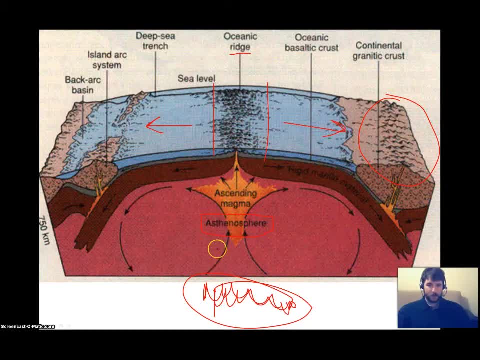 lava lamp. So the lava, the magma underneath the surface it comes up, It gets pushed in either direction when it encounters the rigid mantle And because it's really viscous, it's really thick, it's really gooey, as it goes it's moving the plates with it. So all of the plate boundaries are a result of plate movement And all of those plate movements are a result of those convection currents happening underneath the earth's surface. 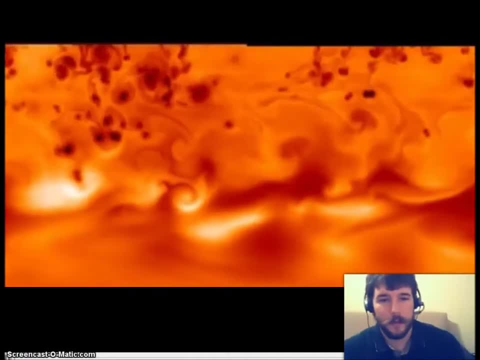 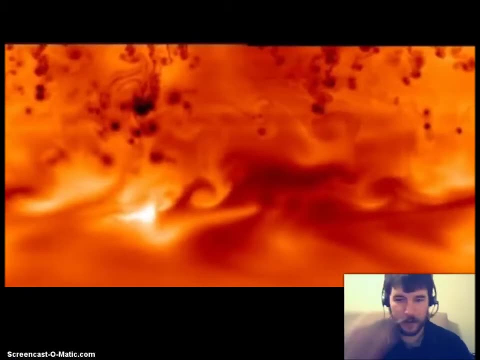 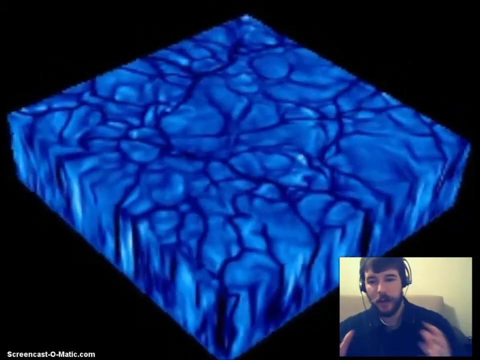 So here is a nice model. You can see the mantle convection driven by heat And you see all these parts that are coming down are showing where the magma has risen up and then drove back down. So here is a nice animation showing you a 3D model of the convection on the earth, well under the earth, And you can see how it sort of looks like water really. 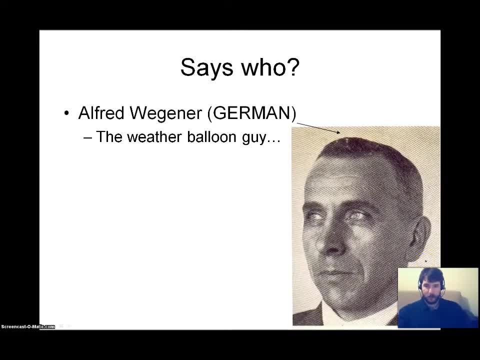 Now this German guy. he's actually the one who invented- you may have heard of it- the weather balloon, Which is, you know, kind of a big deal. Weather balloon, that's Alfred Wegener. He had this whole idea of continental drift. It never really got to be a theory, though that's kind of a bummer. 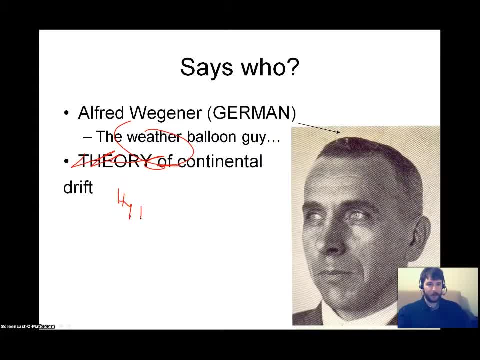 Not a theory, still just a hypothesis, because he could never come up with a really good mechanism. So it was largely untested. in fact it actually got refuted pretty heavily, because he actually thought that these tectonic plates, which are made mostly out of granite and 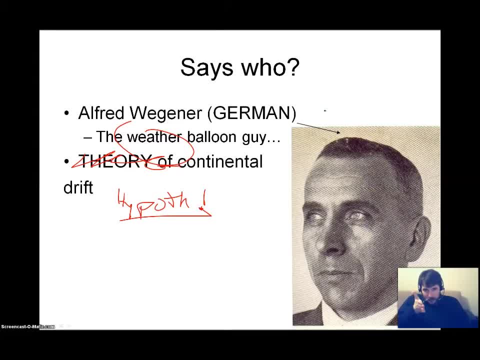 felsic. really low density rocks were actually cutting through the ocean as if they were like a ship, like an icebreaker ship, And the ocean floor is made out of basalt. It's really, really dense and it didn't take physicists long to be like, ah nope, that's not possible. 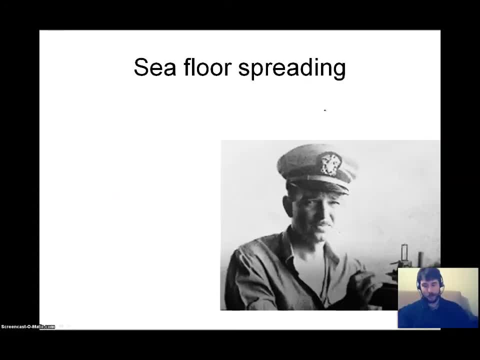 The continental crust would be destroyed, Not going anywhere. And then this guy, Henry Hess- here's his picture There. he is all pretty and Hess-like. He actually came up with this whole idea After discovering the mid-ocean ridge And he published this whole idea later on in the 60s. 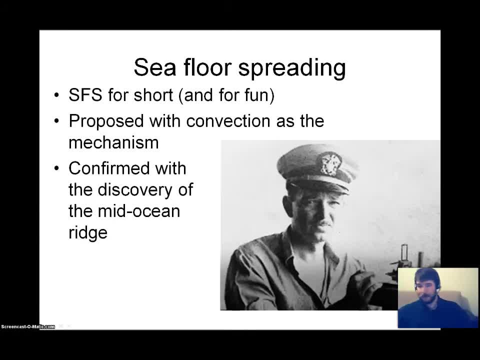 And he actually was able to come up with that whole mantle convection current as the mechanism. So now we have a mechanism to go with the idea and then the scientists are happy. But this didn't happen for a long, long time. Wegener was like way back in the 1910s. 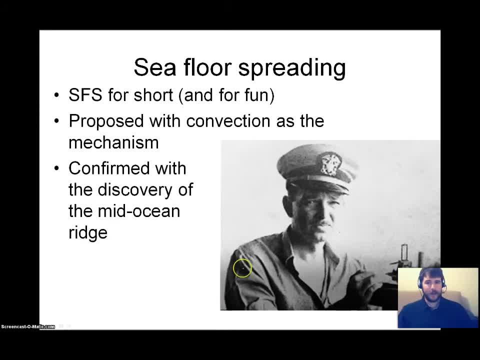 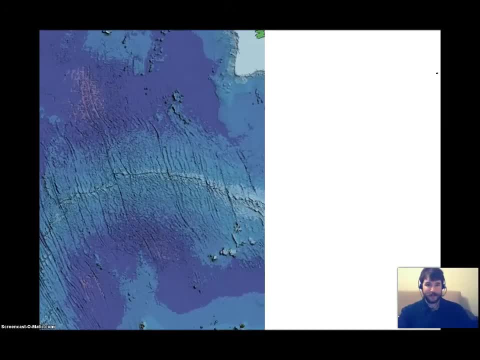 You know he was World War I era. This guy took till World War II and way after the war was over before he finally published it. he published his ideas and it was accepted by the scientific community. So here's a picture actually showing you that. you can see right here the spreading center going right through the middle there. 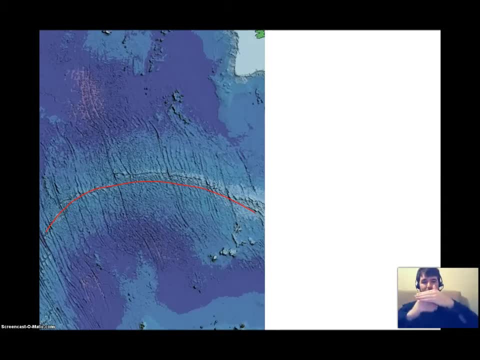 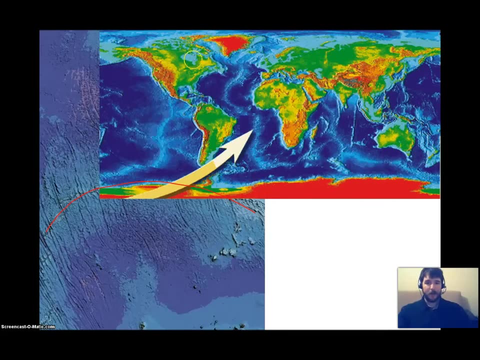 That is our mid-ocean ridge And you can see on either side. it's spreading and it creates all this really beautiful surface topography that we're going to talk more about in class Here. on this map you can see the highlighted blinky areas. 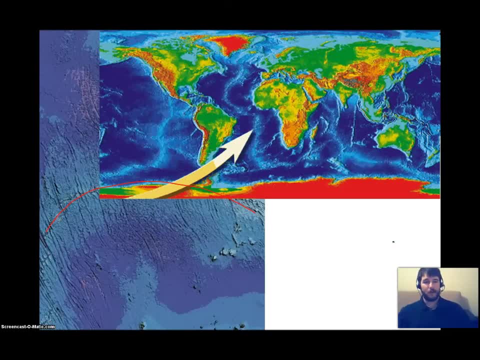 Those are showing you all the different spreading centers in the ocean. These are all mid-ocean ridges. This one right here is the main one, That's the Atlantic mid-ocean ridge. That's the one that Hess discovered, you know, going back and forth here fighting the Germans.